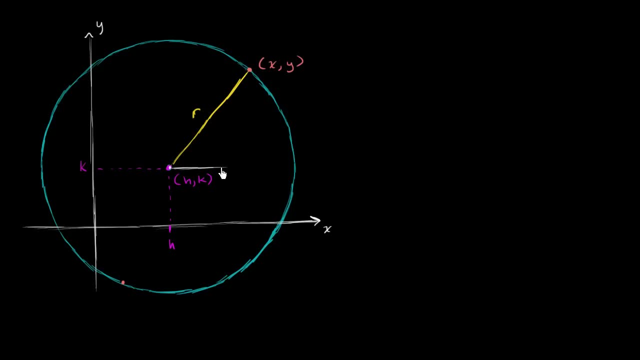 Let's draw one segment that is parallel to the x-axis, going like this. And let's draw another segment, starting at x, y, that is parallel to the y-axis. that's completely vertical. So this one is completely vertical, This one is completely horizontal. 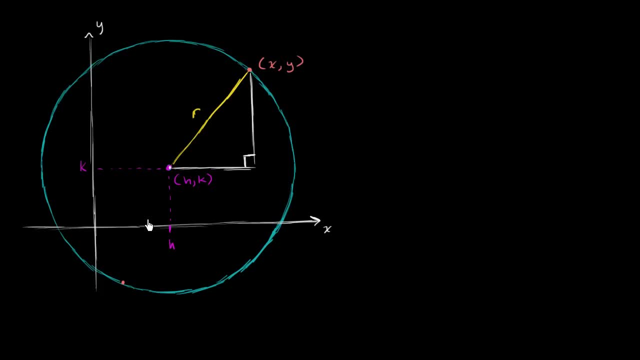 So this is going to be a right angle right over here. So if we can figure out, if we can express the height of this line in terms of the variables we've just put out, and if we can express the height or the width of this line right over here, 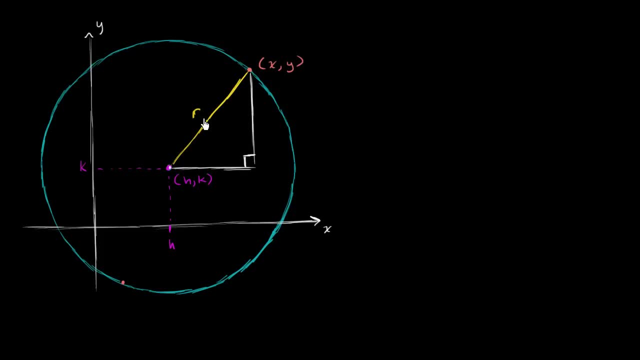 in terms of these variables. somehow, then, we can relate those between that and r using the Pythagorean theorem. r is the hypotenuse of this right triangle. Well, what's this height going to be? Well, we know this point right over here. 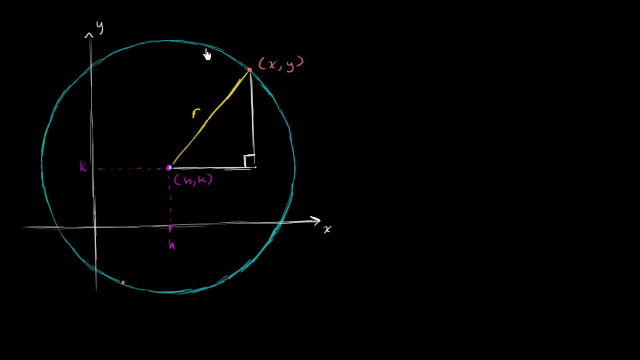 has a y-coordinate of k, This point over here. well, that just has a y-coordinate. I guess we could just say that has a y-coordinate of y. So this distance right over here is going to be the same exact thing as this distance right over. 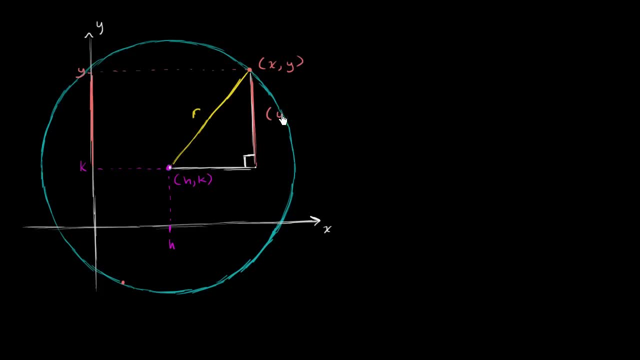 here. So it's going to be y minus y, It's going to be y minus k. and what's this distance going to be? Well, same exact argument, This is h, and this point right over here if we go all the way, or this point on the x-axis. 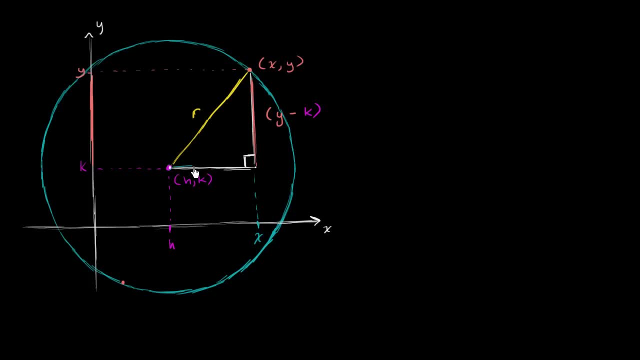 well, we could just call that x. So what's this distance right over here? Well, this distance is going to be x, x minus h. So what is the relationship between this side of length, x minus h, this side of length y minus k and r? 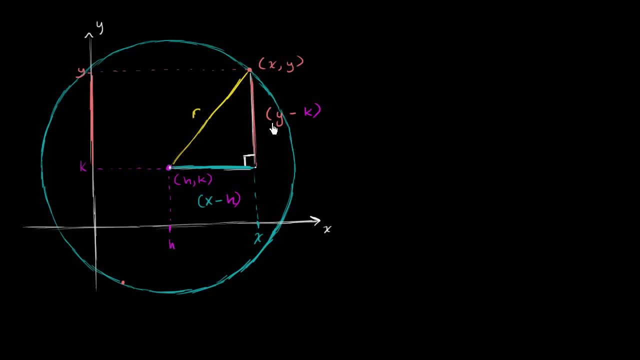 What's the Pythagorean theorem? The sum of the squares of the two shorter sides is going to be equal to the square of the hypotenuse. So one of the shorter sides has length x minus h, so I could write x minus h. 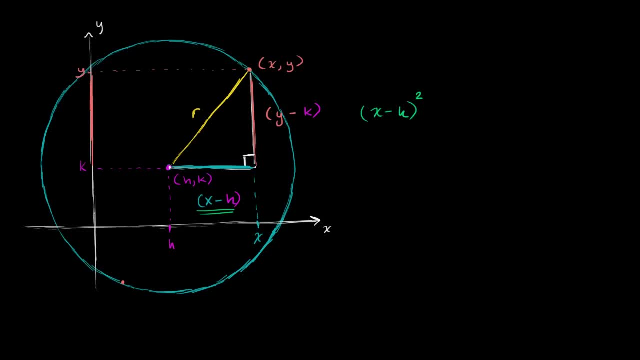 So the length of that side squared plus the length of this side- let me do this in a color that I haven't used yet- plus, All right, the length of this side squared. so plus y, minus k squared is going to be equal to the hypotenuse squared. 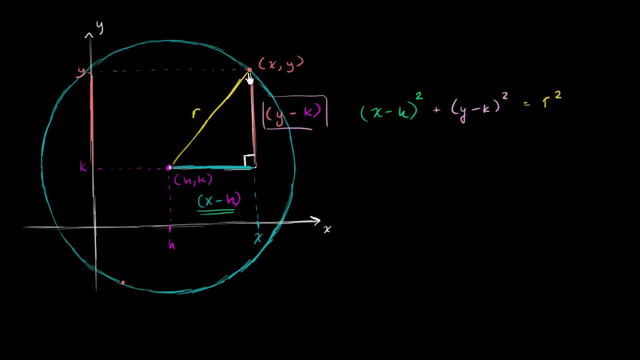 is going to be equal to the radius squared. And just like that we have found the general equation of a circle where h comma, k is the center of the circle and r is the radius. Any combination of x's and y's that meet this. 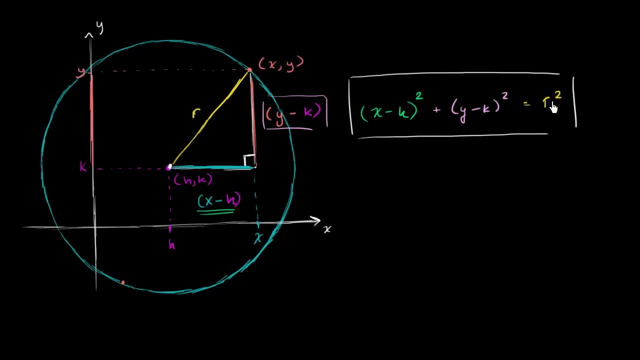 for which this is true. given your center, given h and k and given the radius, then any x's and y's that will meet these constraints are going to be on the circle. So another way you could think about it. if someone said: 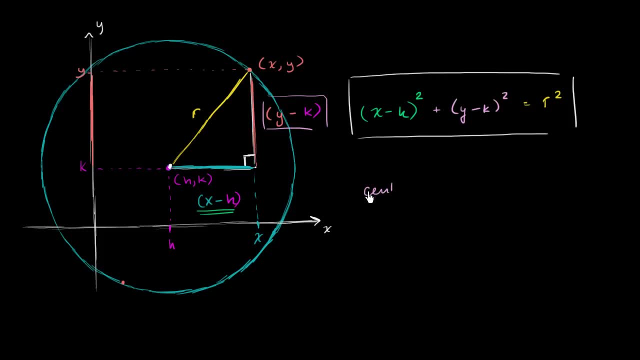 hey look, I have a center, The center. let me write it this way: the center of my circle is at the point I don't know, 5.. 5, negative 5.. And if they said that the radius is equal to 4,? 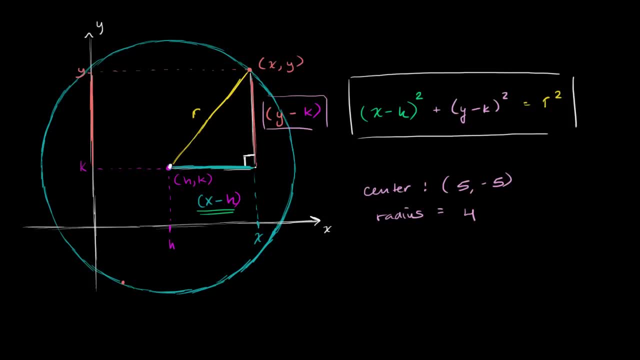 then we could immediately say what the equation of the circle is going to be. It's going to be x minus this right over here. Let me color code this a little bit: This right over here is our h, That's our h. This right over here is our k. 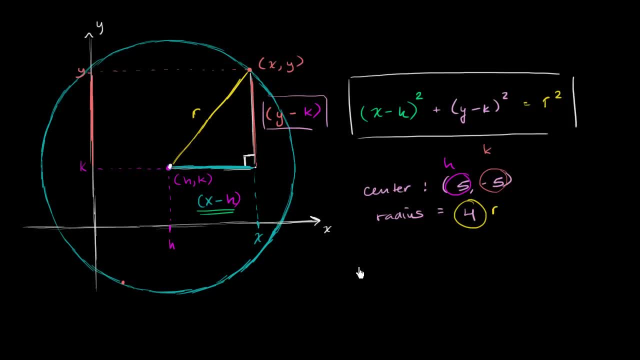 And this is our radius. This right over here is our radius. So the equation of the circle would be x minus h. so x minus 5 squared plus y minus k, k is negative 5.. So if you subtract negative 5, that'd. 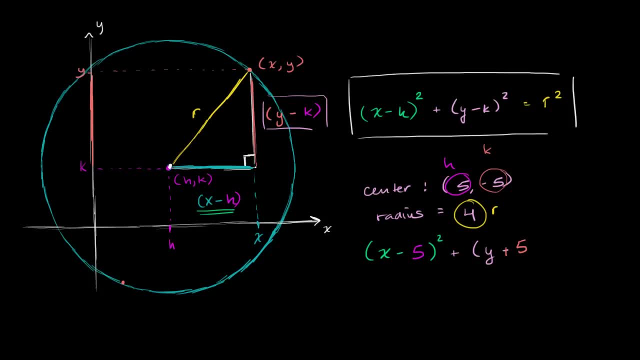 be the same thing as adding positive 5.. So y plus 5 squared is equal to r squared. Well, r in the example I just showed is equal to r. squared I just made up is equal to 16.. So if someone told you that the center is at 5, negative 5,. 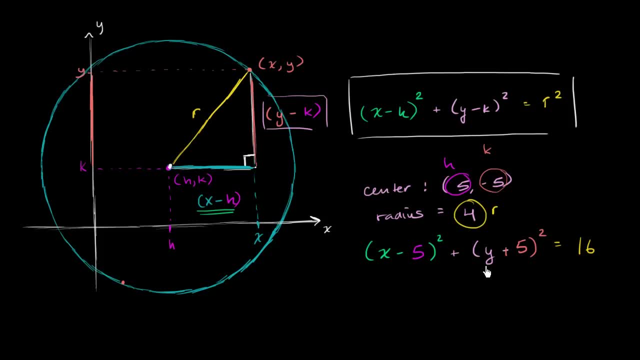 the radius is 4,. well, this is going to be the equation of the circle. On the other hand, if someone gave you this as the equation of the circle, you know that the center is going to be at 5.. It's going to be at x equals 5 and y equals.